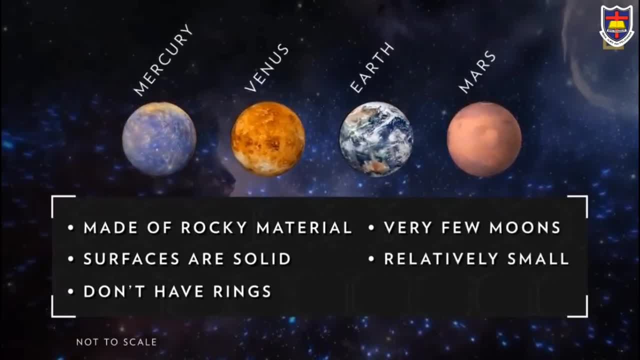 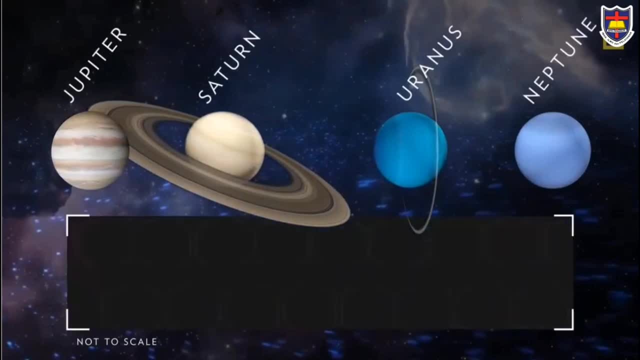 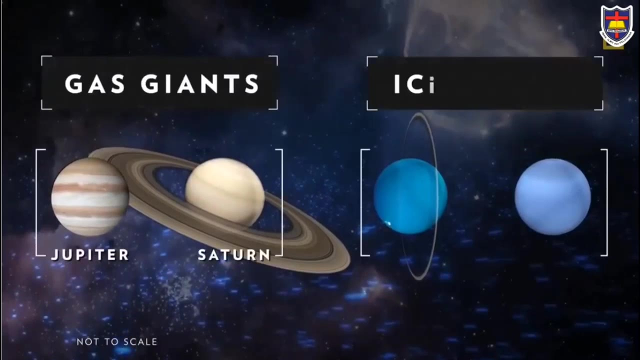 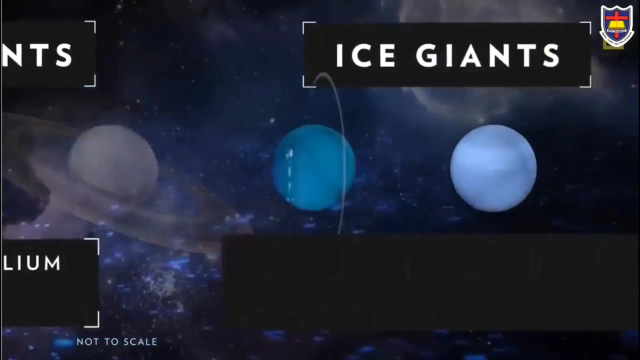 They have a very few or no moons And they are relatively small. The jovian planets include gas giants Jupiter and Saturn, and ice giants Uranus and Neptune. The gas giants are predominantly made of helium and hydrogen, And the ice giants also contain rock ice and a liquid mixture of water, methane and ammonia. 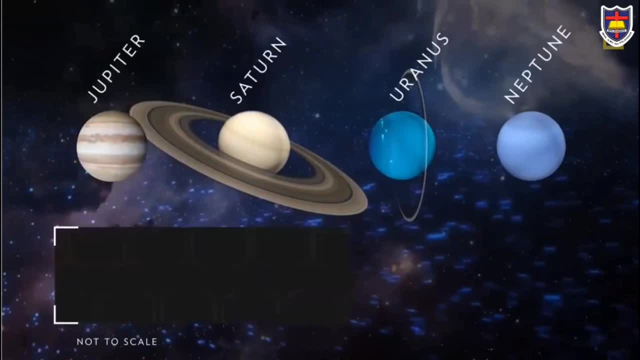 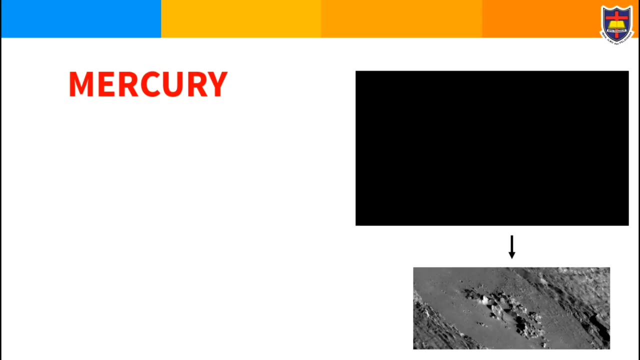 All four jovian planets are made of rock ice and a liquid mixture of water, methane and ammonia. The jovian planets have multiple moons, support a ring system, have no solid surface and are immense. The first planet is Mercury. 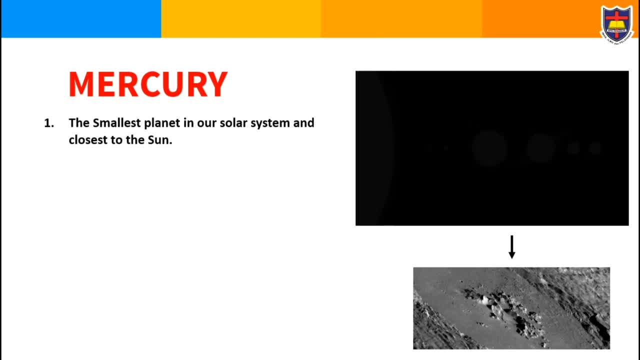 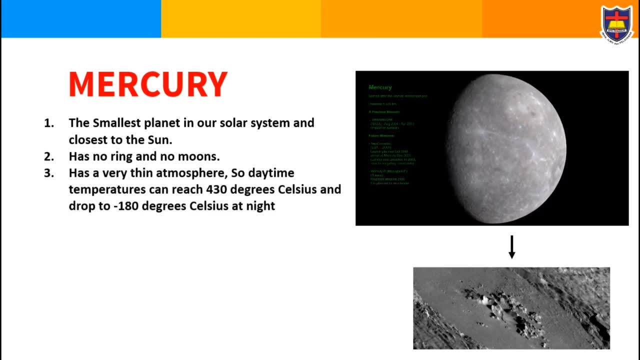 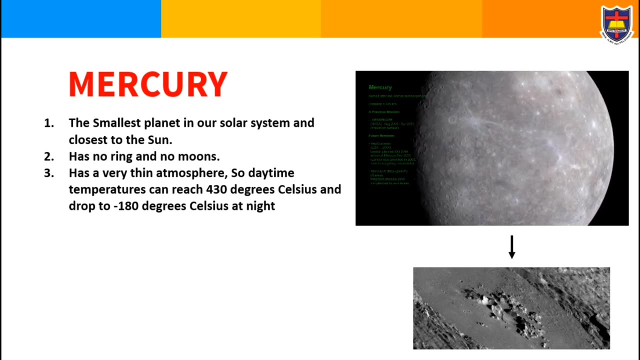 Mercury is the smallest planet in our solar system and the closest to the sun. There are no rings around Mercury. Mercury has no moons. Mercury has a very thin atmosphere, so atom temperatures can reach 430°C and drop to minus 180°C at night. 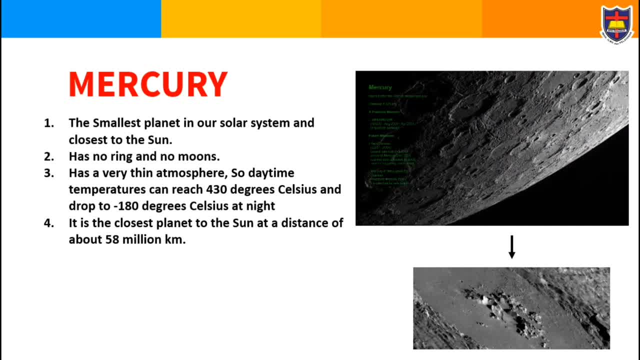 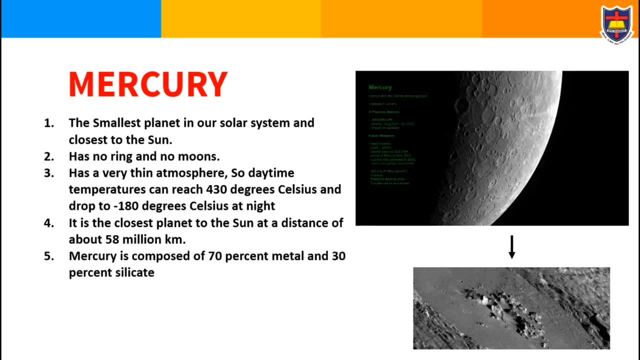 It is the closest planet to the Sun, at a distance of about 58 million kilometers. Mercury is composed of 70% metal and 30% silicate. Mercury makes a complete orbit around the Sun In just 88 Earth days. The second planet is the Venus, the hottest planet in our solar system. 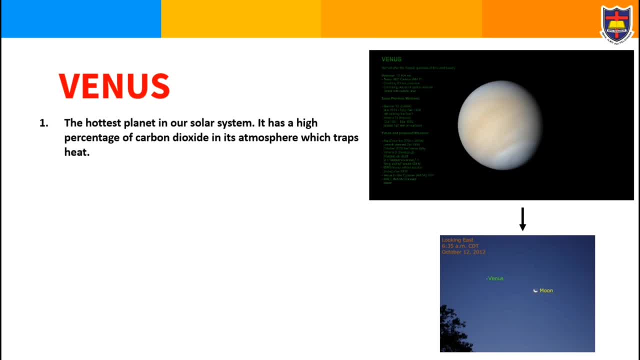 It has a high percentage of carbon dioxide in its atmosphere, which traps heat. Venus is the brightness of all planets in the night sky and also called the morning and evening star, as it appears in the eastern sky before sunrise and in the western sky after sunset. 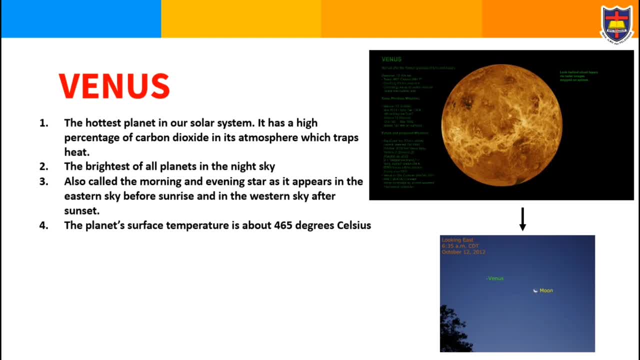 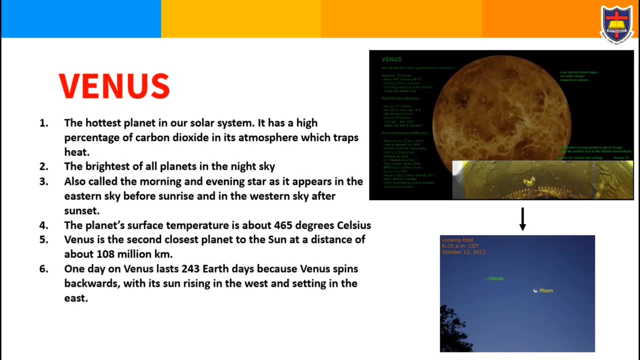 The planet's surface temperature is about 465°C. Venus is the second closest planet to the Sun, at a distance of about 108 million kilometers. One day on Venus lasts 243 Earth days, because Venus spins backward, with its sun rising in the west and set in the east. 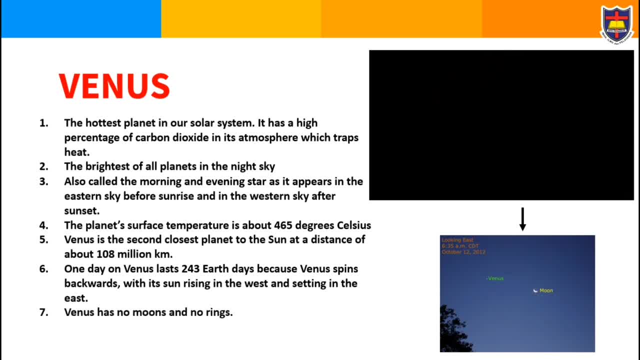 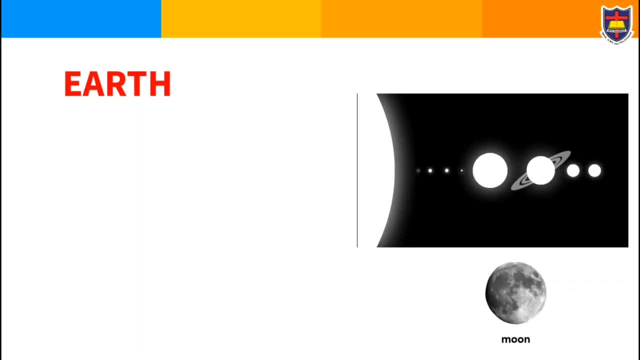 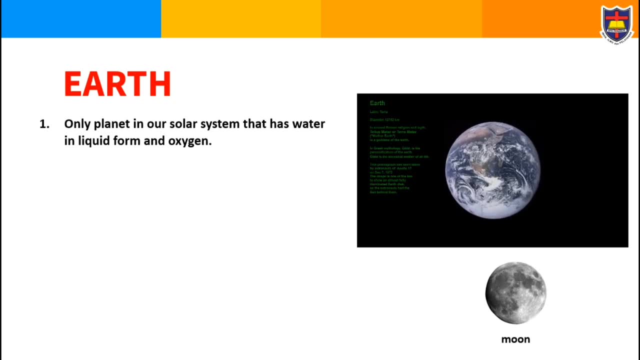 Venus is called Earth's twin. The reason for that is because Venus has no rings. The third planet is Earth, Only planet in our solar system that has a water in liquid form and oxygen, so it means supports life. Earth makes a complete orbit around the Sun in about 365 days. A day on Earth is 24 hours. 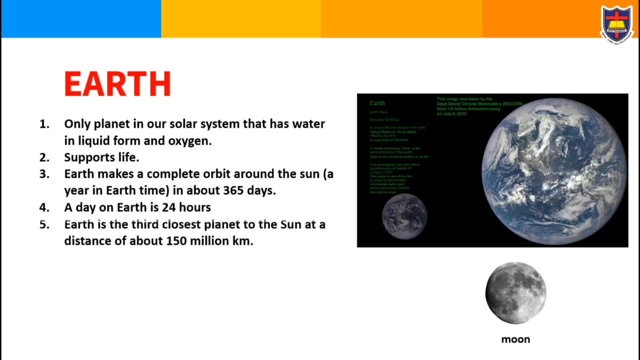 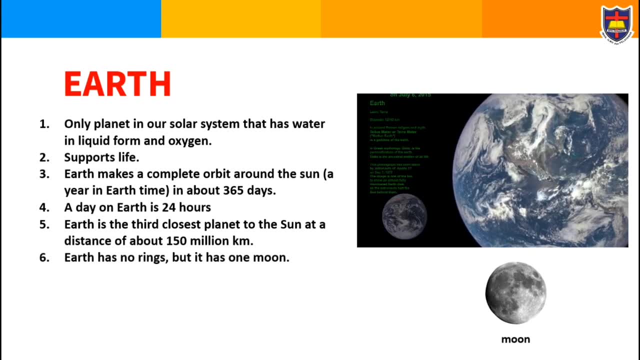 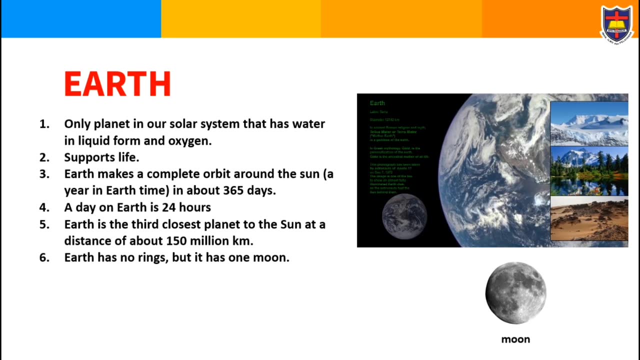 Earth is the third closest planet to the Sun, at a distance of about 150 million kilometers. Earth has no rings, but it has one moon. The moon orbits the Earth like the Earth orbits the Sun. Earth's atmosphere is 78% nitrogen, 21% oxygen and 1% other ingredients. 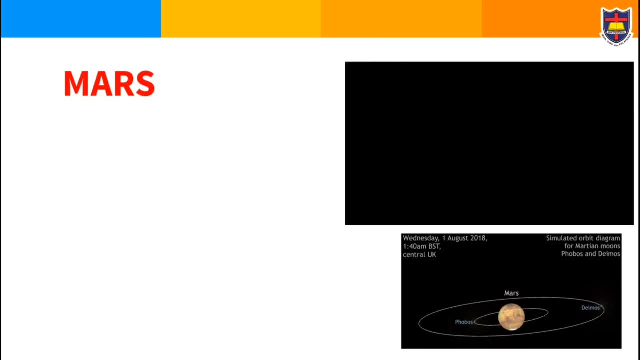 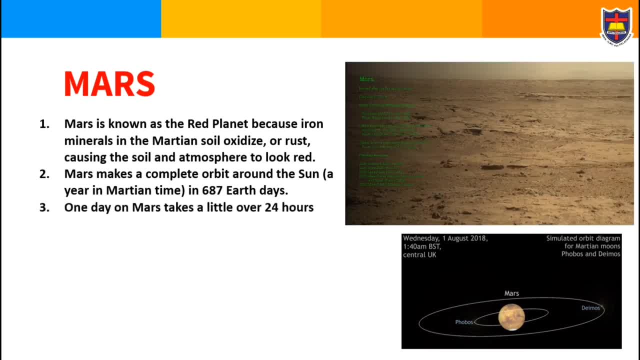 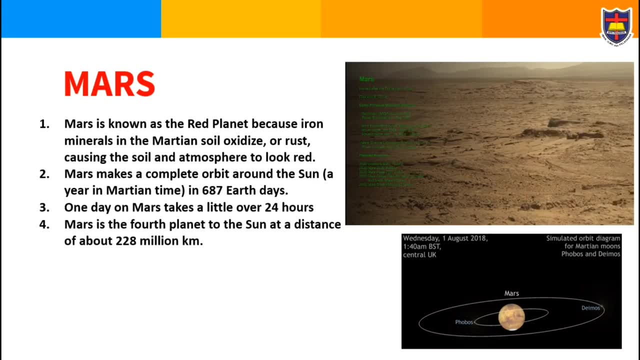 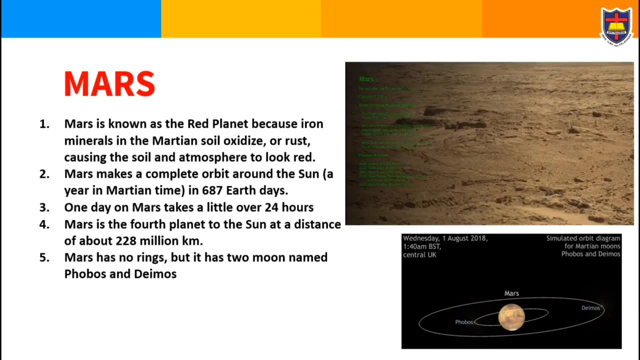 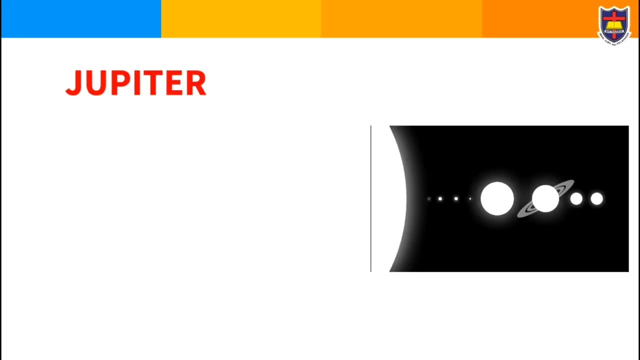 One day on Mars takes a little over 24 hours. Mars is four planets to the Sun, at a distance of about 228 million kilometers. Mars has no rings, but it has two moons named Probus and Deimos. Okay, guys, guess what? 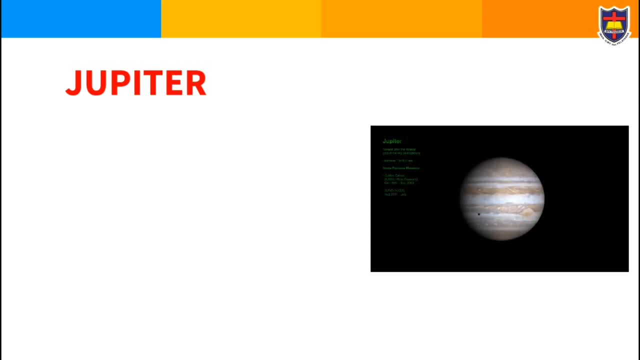 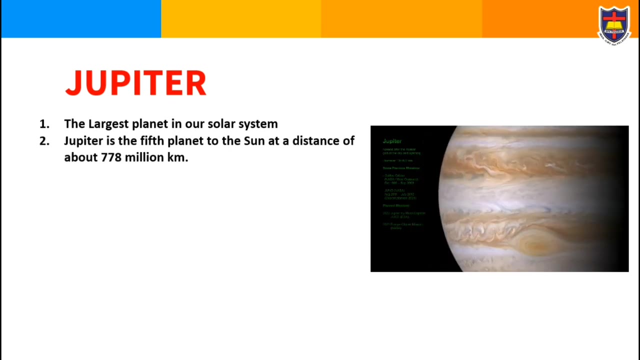 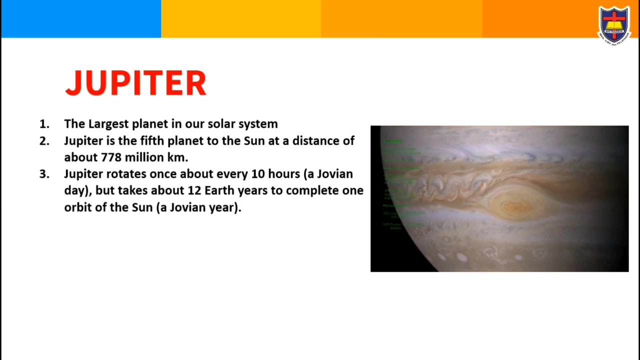 What's next? Yeah, correct, Jupiter The fifth planet is Jupiter, the largest planet in our solar system. Jupiter is the fifth planet to the Sun, at a distance of about 778 million kilometers. Jupiter rotates once about every 10 hours, but takes about 12 Earth years to complete. 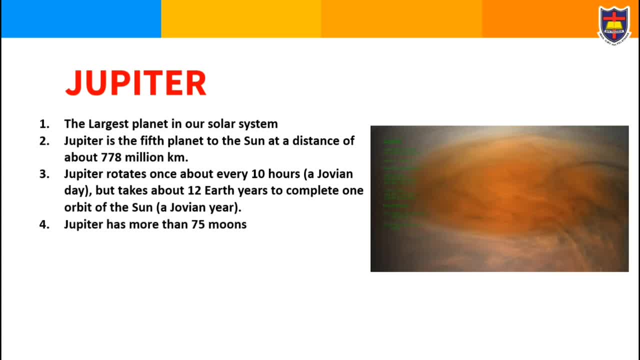 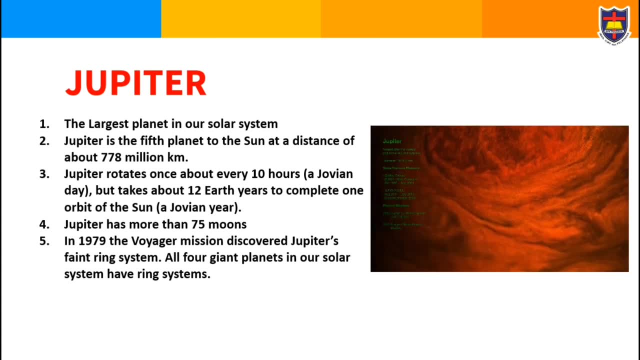 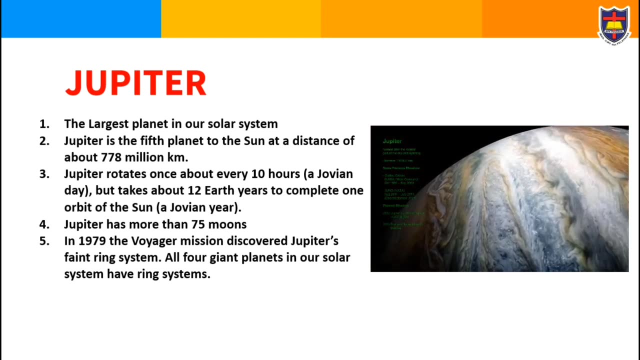 one orbit of the Sun. Jupiter has more than 75 moons. In 1977, Jupiter was the fifth planet to the Sun. In 1979, the Phaedra giant fusion discovered Jupiter's faint ring system. All four giant planets in our solar system have ring systems. 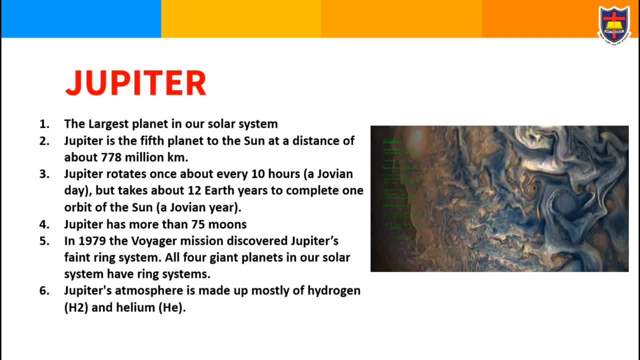 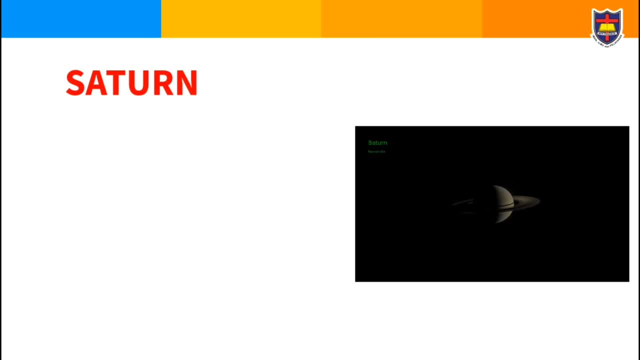 Jupiter's atmosphere is made mostly of hydrogen and helium. Okay, now the yellow is the planet. yeah, Saturn, the second largest planet in our solar system. Saturn has the most sphincter ring system that it has on Mars, like only one. 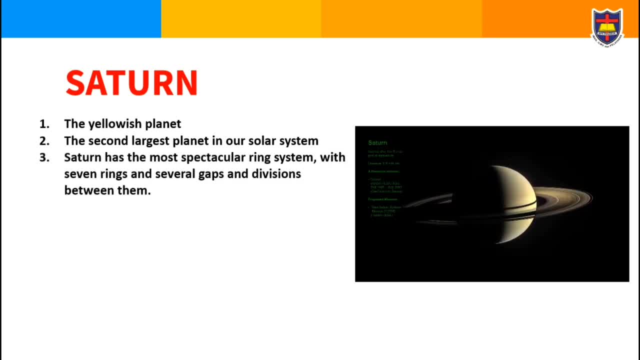 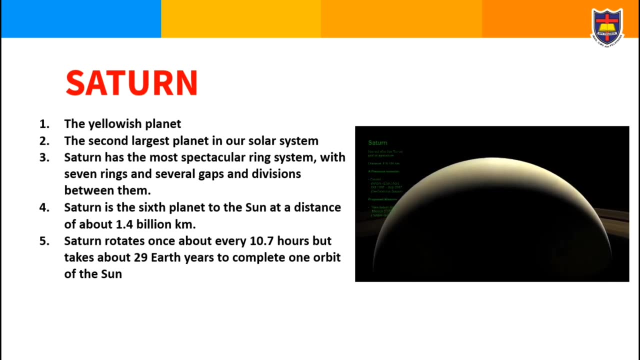 Comes in with a unique, uniqueling. Look at that Venus system with seven rings and several gaps and divisions between them. Saturn is the sixth planet to the Sun, at a distance of about 1.4 billion kilometers. Saturn rotates once about every 10.7 hours, but takes about 29 Earth years to complete. 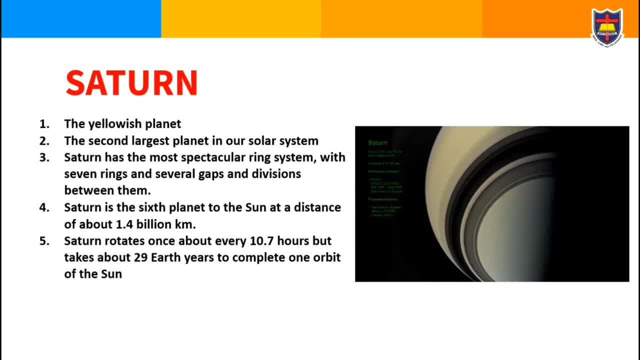 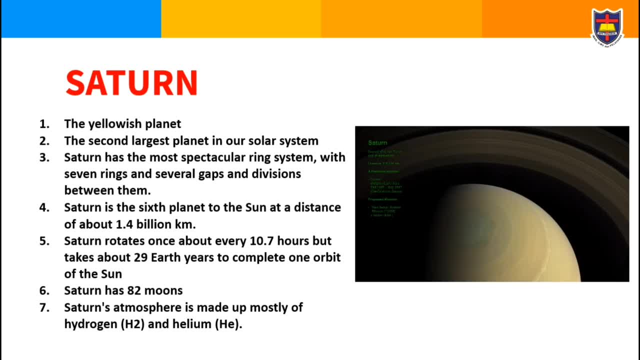 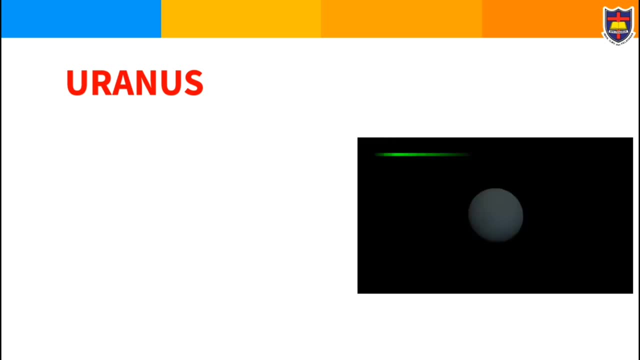 one orbit of the Sun. Saturn has 82 moons. Saturn's atmosphere is made up mostly of hydrogen and helium. Okay, guys, the seventh planet is Uranus, the name-like hero in Mobile Legends, right, Okay? Uranus is about four times wider than Earth, the third-largest planet in our solar 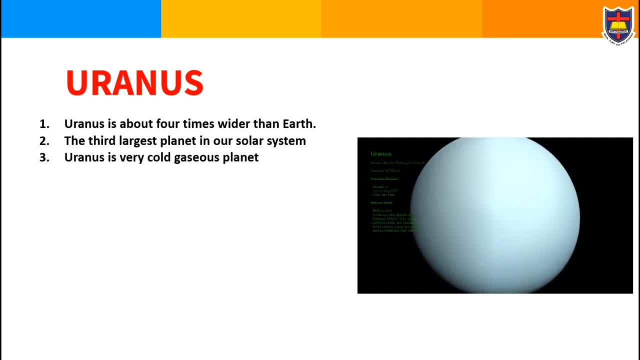 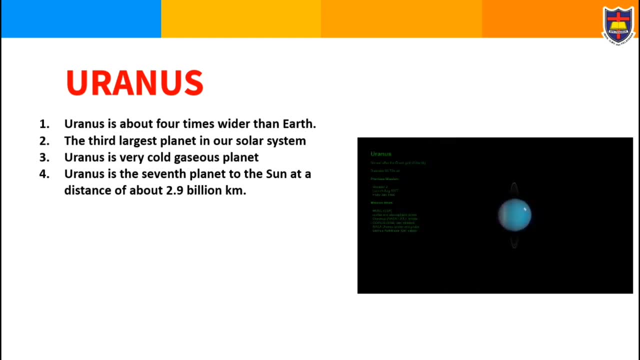 system. Uranus is a very cold-gaseous planet. Uranus is the seventh planet to the Sun, at a distance of about 2.9 billion kilometers. Uranus rotates once about every 17 hours, but takes about 84 Earth years to complete. 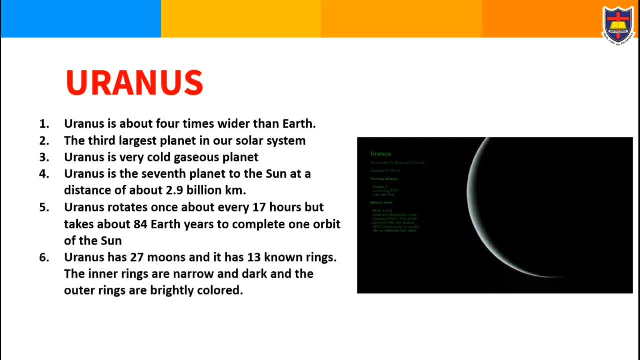 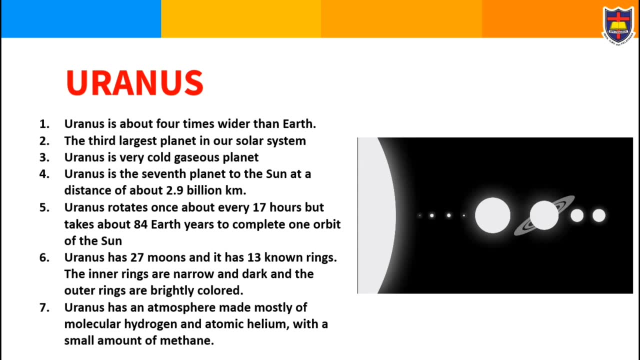 one orbit of the Sun. Uranus has 27 moons and it has 13 known rings. The inner rings are narrow and dark and the outer rings are brightly colored. Uranus has an atmosphere made mostly of molecular hydrogen and atomic helium, with a small amount.